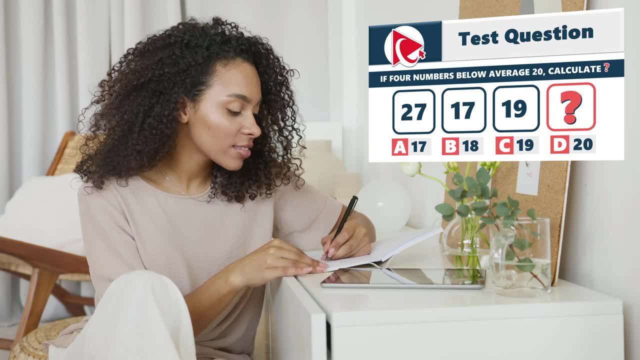 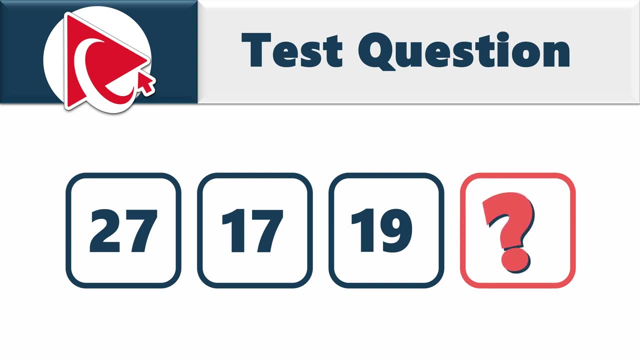 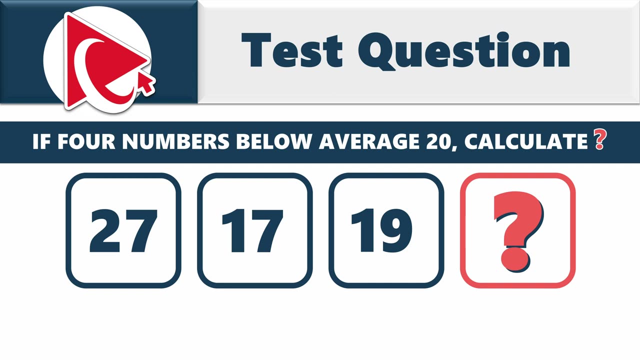 knowledge and refine your approach, paving the way for stronger performance in the future. You are presented with four numbers. In fact, the fourth number is missing And the question is if four numbers below average 20, you need to calculate the missing number. Once calculated, 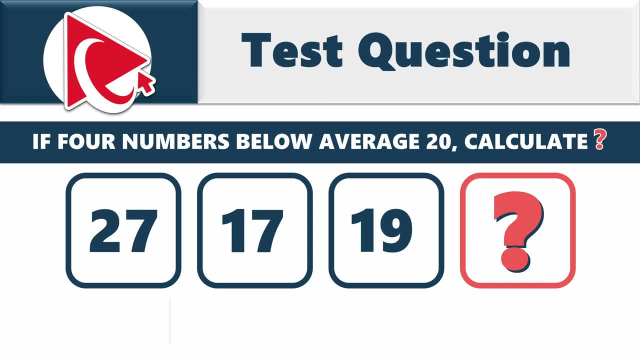 you need to select the answer out of four possible choices: Choice A: 17.. Choice B: 18.. Choice C: 19. And choice D: 20.. Are you having doubts about this question? Don't worry, It's natural to. 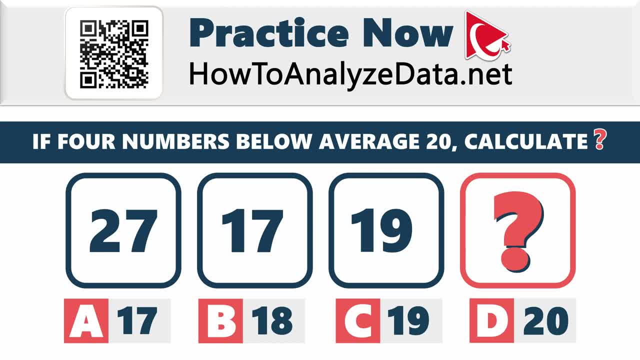 encounter challenges. I feel like I'm going to be able to solve this question in a few minutes. I feel exactly the same way, But remember, every problem has a solution And I believe you will find it with your ingenuity and perseverance. Let's tackle it as a team. 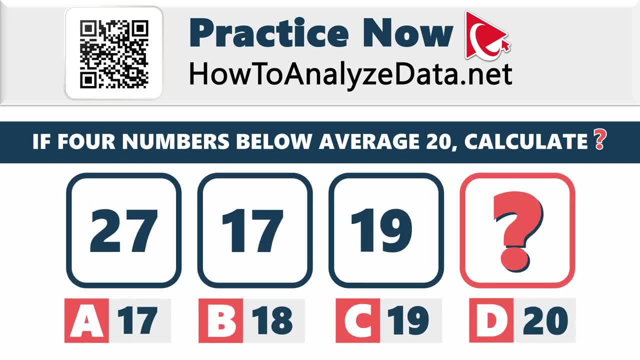 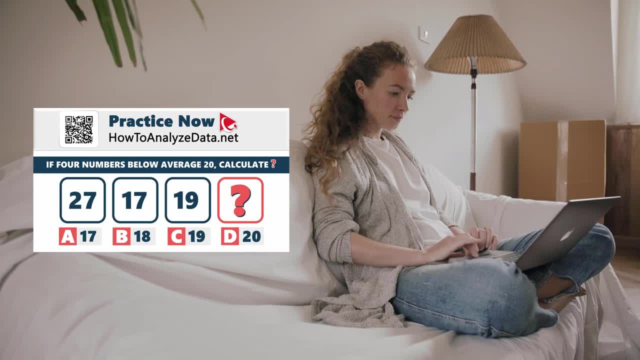 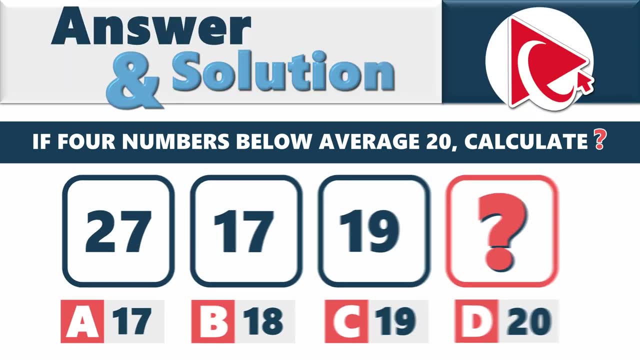 Are you ready to present your solution? Let's start exploring and see where our paths converge And if uncertainty creeps in, stay positive. Every question tackled, regardless of the outcome, contributes to a better future, And the solution here might be easier than you think. If four numbers average 20,. 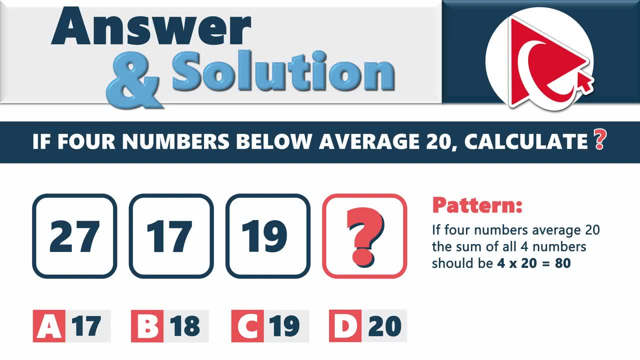 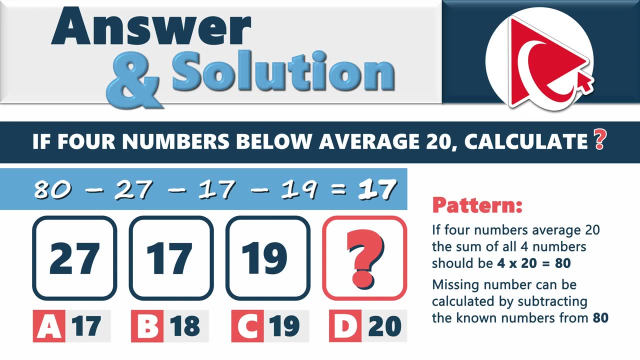 the sum of all four numbers should be 4 multiplied by 20 and equals 80.. The missing number can be calculated by subtracting no numbers from 80. So the missing number can be calculated as 80 minus 27, minus 17, minus 19, and equals 17.. So the correct answer here is choice A, 17.. 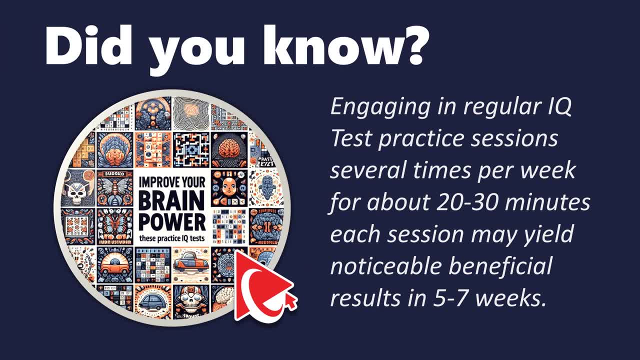 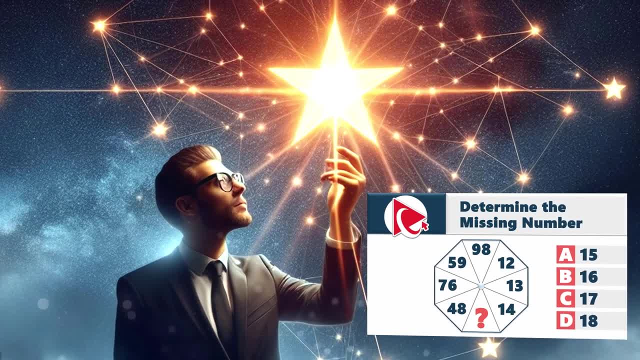 When you look at this question, you have to realize that when you answer it it would feel like adding a shining star into the constellation of your success. So keep shining bright. You're presented with octagon. It has numbers inside. There are seven numbers and the eighth number. 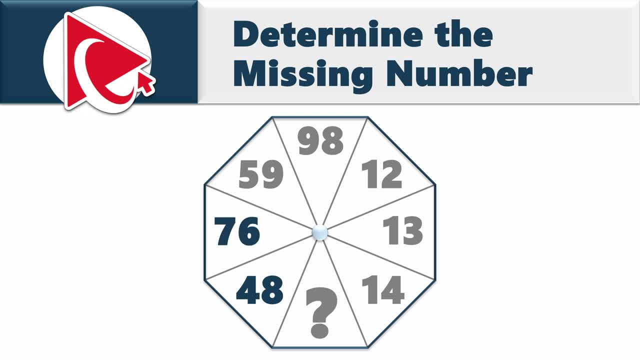 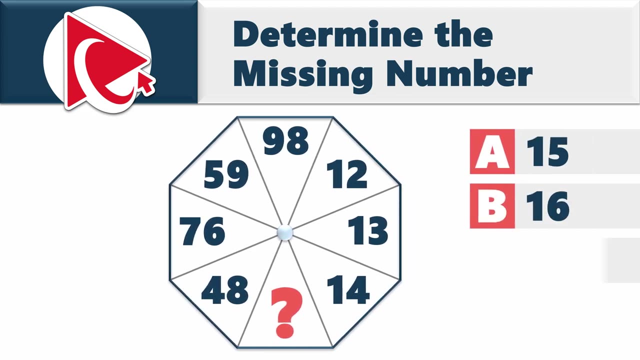 is missing. The numbers are 48,, 76,, 59,, 98,, 12,, 13,, 14.. And then comes the missing number which you need to select out of four. So you choose A, 15. You choose B, 16. You choose C, 17.. You choose D: 18.. I hope you noticed there. 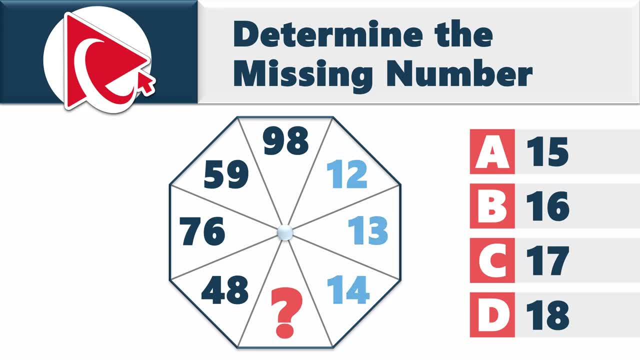 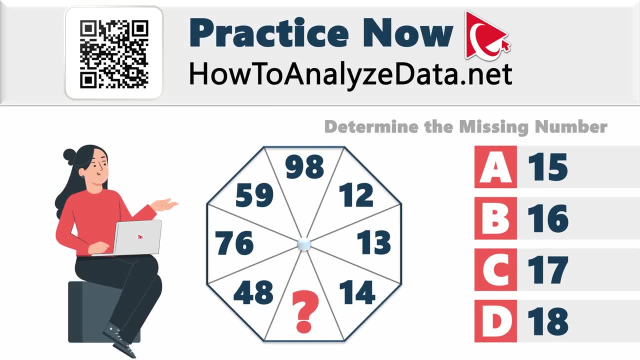 is a pattern here. Look at 12,, 13,, 14, or maybe not. You think it's a tricky question. Fear not, You're in a good company on this quest, Whether you're a seasonal problem solver or just starting. 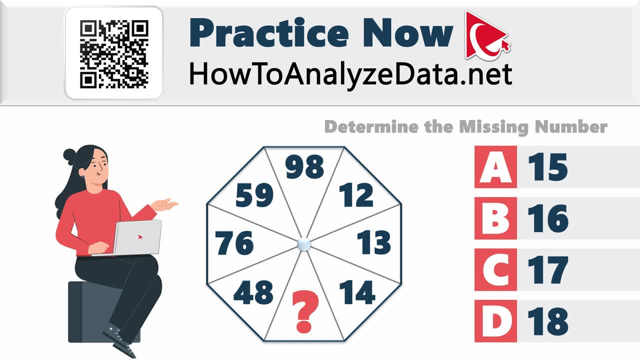 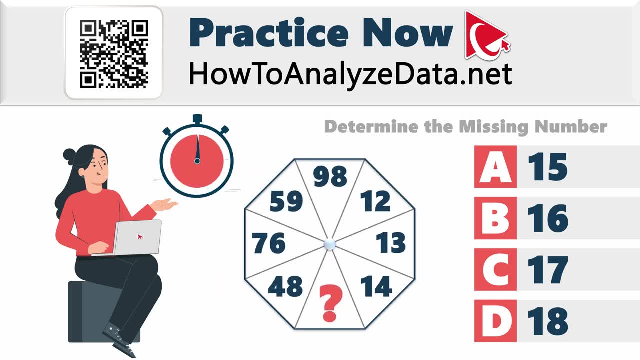 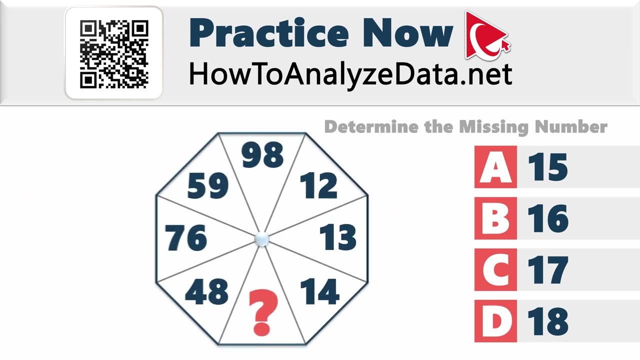 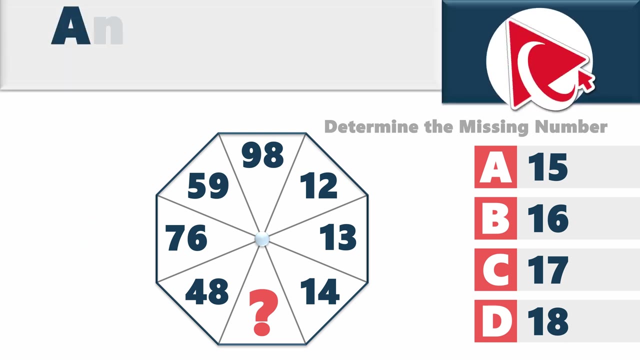 out. I have confidence in your abilities. Pause for a moment, channel your inner creativity and let's conquer this challenge side by side is just around the corner. are you prepared with your solution? i am curious to compare notes, so let's move forward and share our answers. to answer this question, you need to look closely. 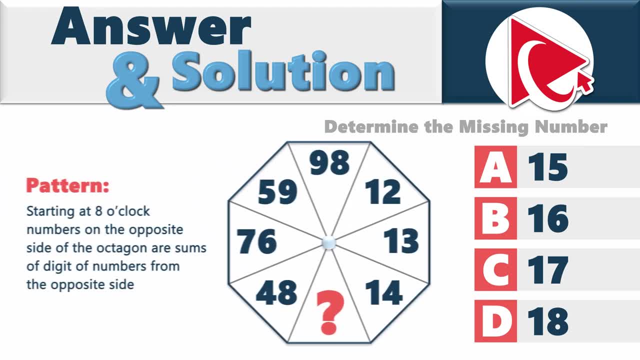 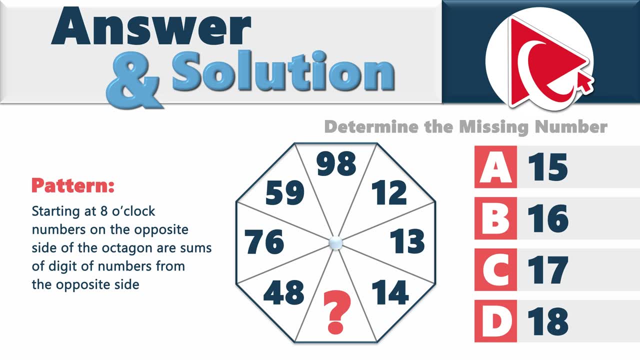 to determine the pattern. and the pattern here is that, starting at eight o'clock, numbers on the opposite side of the octagon are sums of digits, of the numbers from the opposite side. let's look at the example. you see the number 48 at 8 o'clock. 4 plus 8 equals 12, and that's exactly the number. 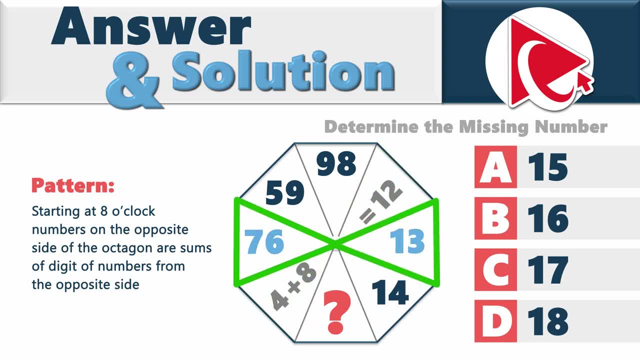 on the opposite side. let's keep looking: 76 converts into 7 plus 6 and equals 13.. 59 converts to 5 plus 9 and equals 14, and then the missing number can be calculated as 9 plus 8 and equals. 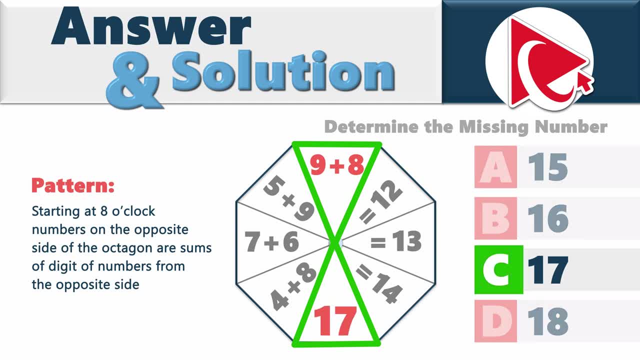 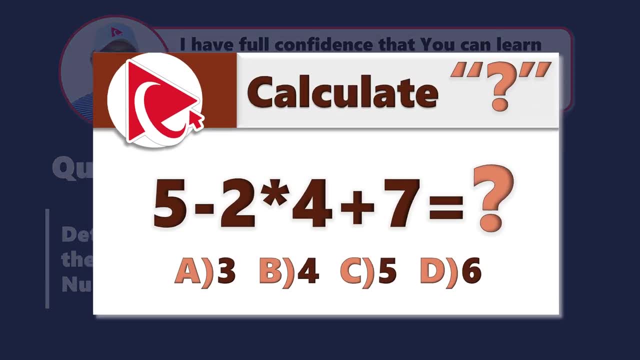 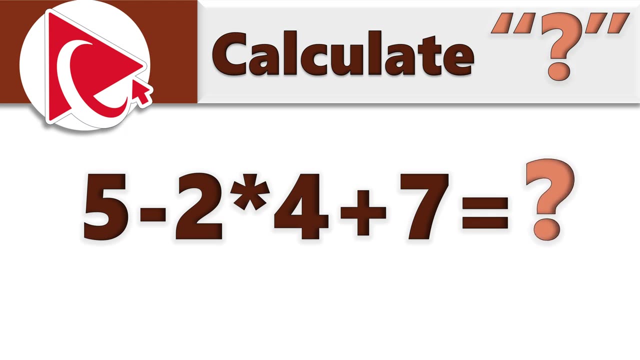 17.. so the correct answer here is choice c 17.. get ready for a mind-bending question that will make you question your own existence. well, maybe not to that extreme, but definitely a cognitive workout. you are presented with the very simple expression 5 minus 2 multiplied by 4 plus. 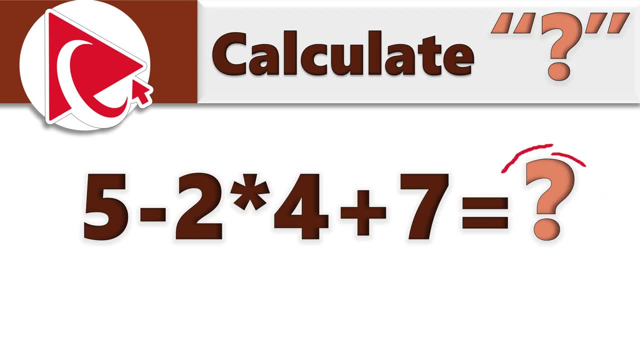 7 equals question mark, and question mark is the value that you need to calculate. once calculated, select your answer out of four possible choices: choice a, three, choose b, four, choice c, five and at least choice d, six. i'm going to give you a hint. make sure to verify your answer before you move. 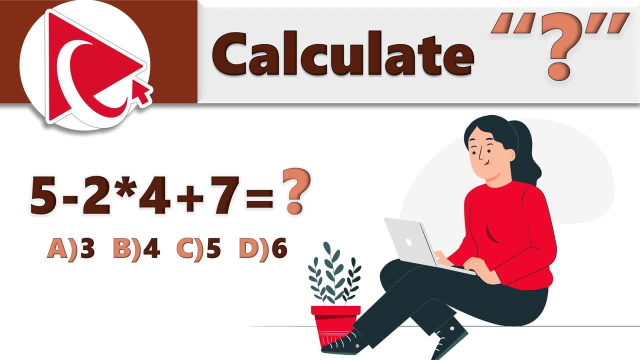 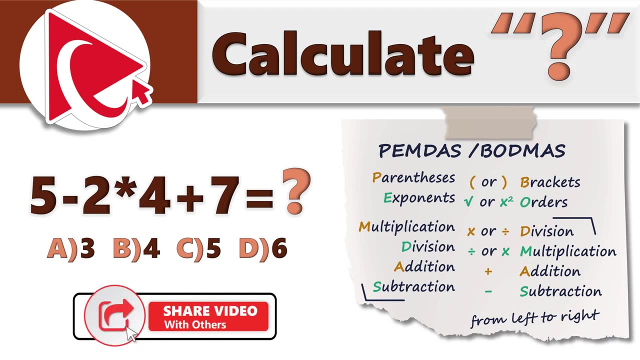 forward. are you ready? let's go ahead and dive into this brain teaser together and remember if you end up calculating a better way to solve it. please share your answer in comments. the key to solve this challenge is to determine the order of operations. you might have heard the term. 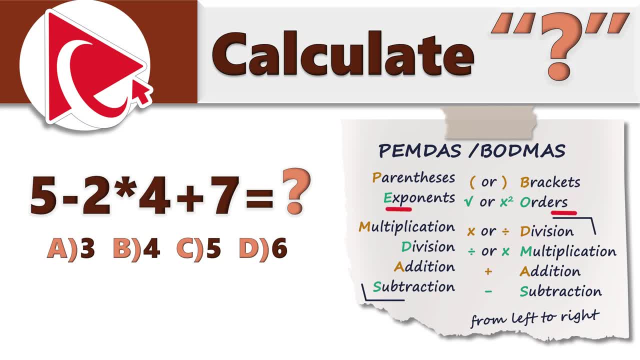 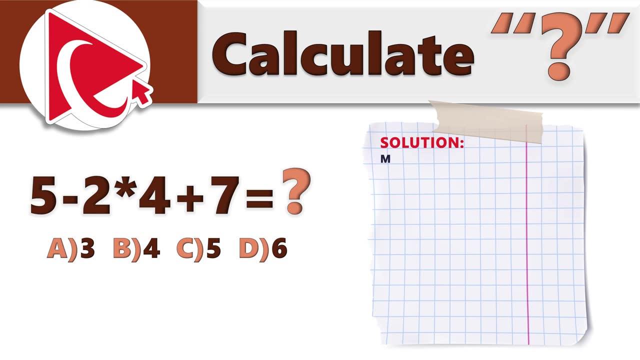 pamdas, which stands for parentheses, brackets, exponents, orders, multiplication, divisions, addition and subtraction, which is also known as bandas, and represents correct way to perform calculations. let's apply this order to this expression. we first need to do multiplication: 2 multiplied by 4 equals 8.. so the updated expression will be 5 minus 8 plus 7.. 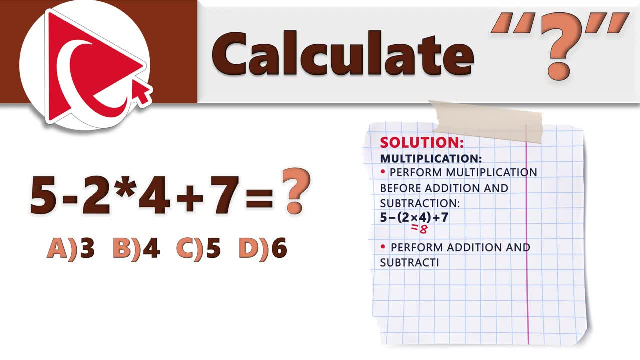 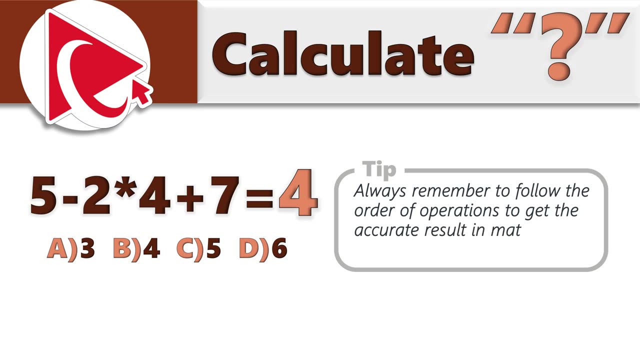 the next operation is from left to right. we need to do subtraction: 5 minus 8 equals minus 3.. minus 3 plus 7 equals 4.. so the tip here is always remember to follow the order of operation to get the accurate result in mathematical calculations. the correct answer here is choice b, 4. 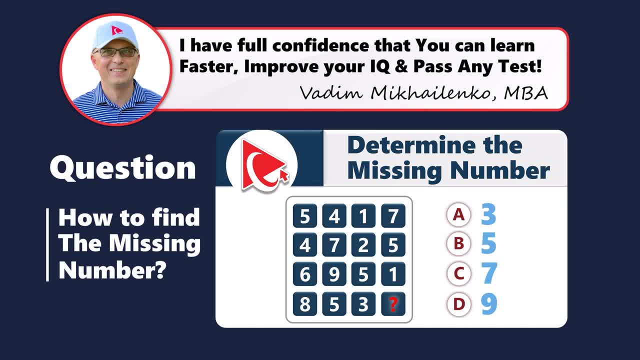 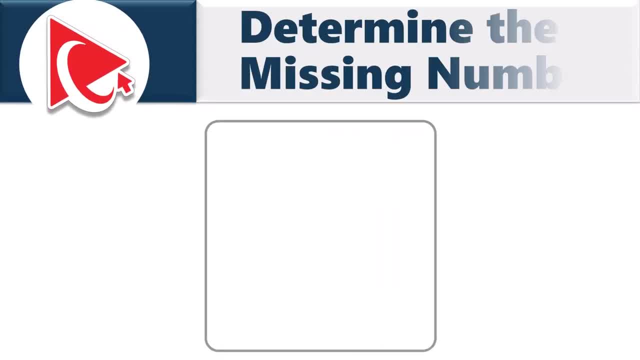 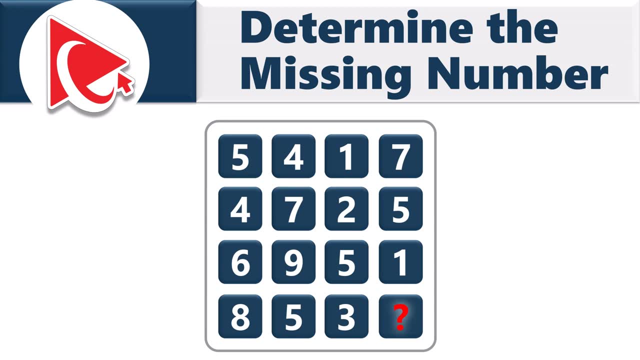 after i saw this question, it reminded me the old phone keypad, but solving it may not be as easy as pushing buttons on this old phone. you're presented with the square- large square has smaller squares where you need to press both hands and former steps. sometimes you need to move the keypad. 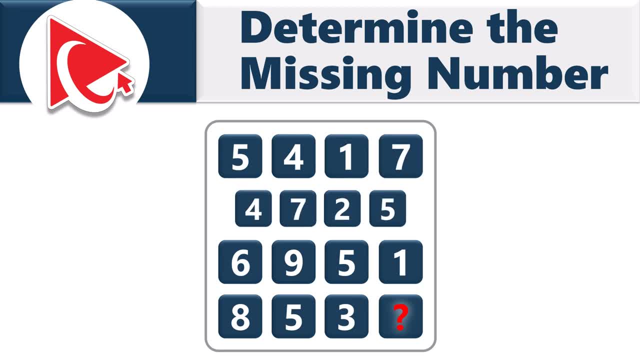 the same way, you need to change the keypad because certain addresses there exist and many things that can work when used differently, and this is exactly the point we will discuss later. alright, let's move it up five to six together, and right now, here's the point, the first two. 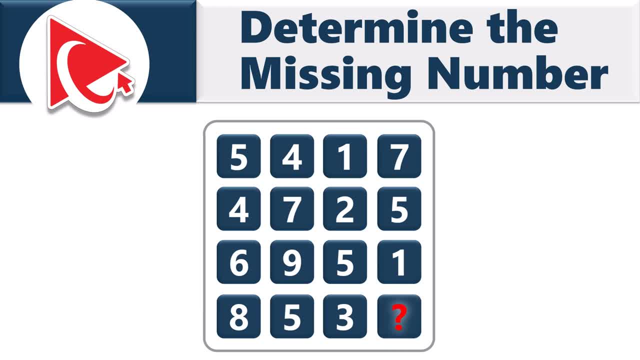 steps you should do is same as before, with the first, in order to go ahead and try to solve both choices. i want you to remember why you're going to learn how to do it this wayowałim. let's move it to the next up. that's it. 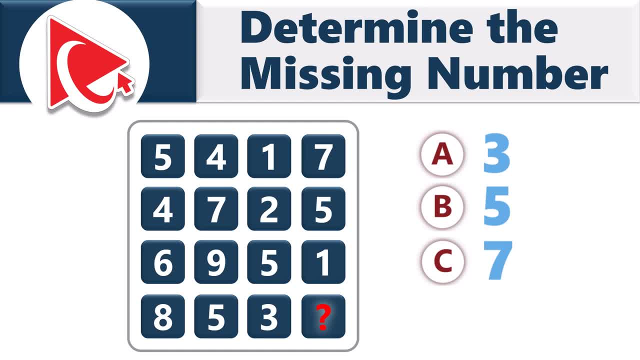 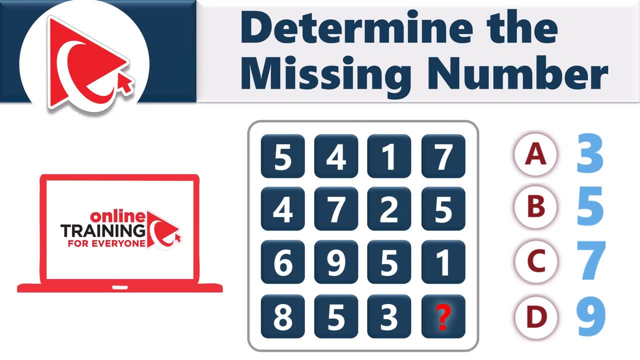 let's do it: 5., 6., 7., 8., 9., 10., 11., 12., 13., 14., 15., 16., 17., 18., 19., 20.. 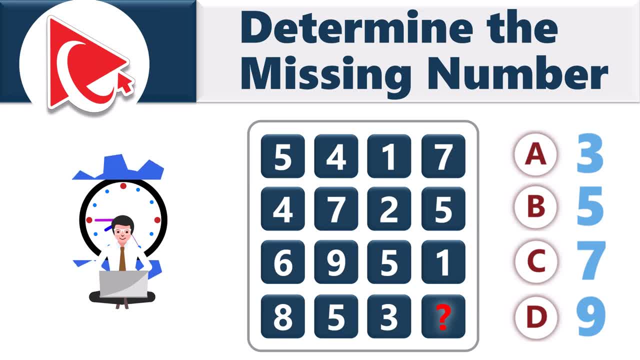 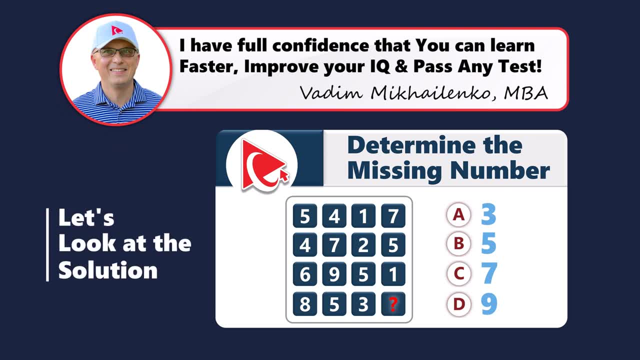 21., 22., 23., 24., 25., 26., 27., 28., 29., 30., 31., 32., 33., 32., 33., 34., 35.. 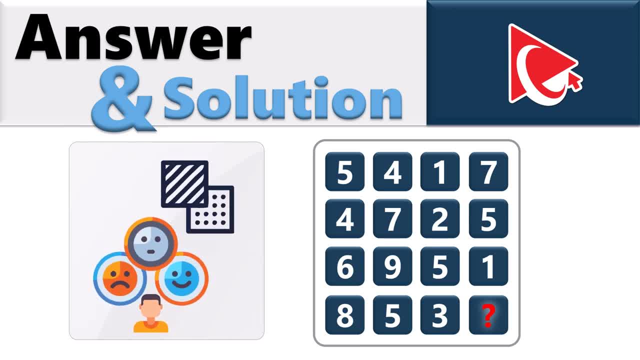 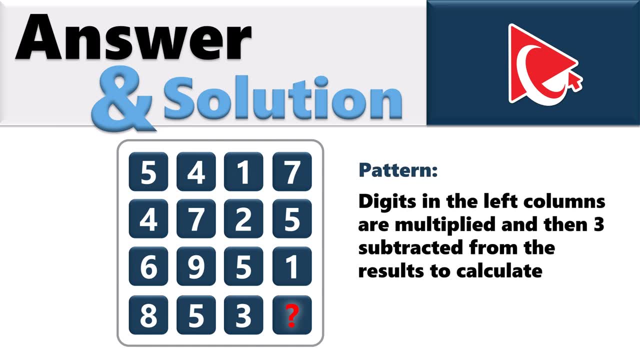 36., 37., 38., 39., 40., 41., 42., 43., 44., 45., 46., 46., 47., 48., 49., 50., 51.. 52., 53., 54., 55., 56., 57., 58., 59., 60., 61., 62., 63., 62., 63., 64., 65., 66.. 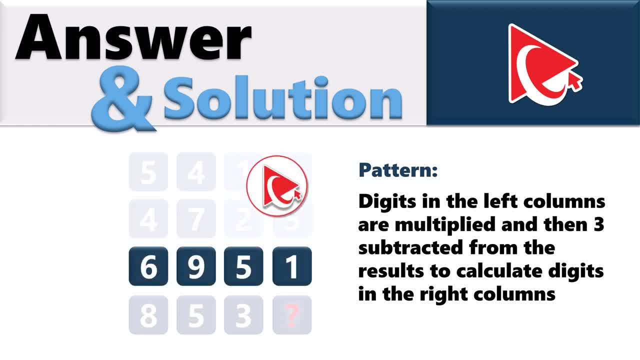 67., 68., 67., 68., 69., 69., 70., 71., 71., 72., 72., 73., 73., 74., 74., 75., 76.. 77., 78., 78., 79., 79., 80., 80., 81., 81., 82., 82., 83., 83., 84., 84., 85., 85.. 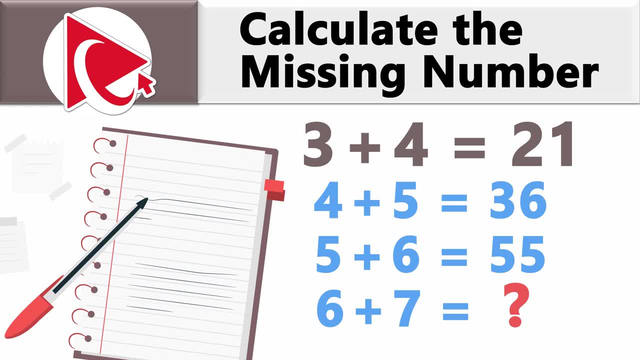 86., 86., 87., 86., 87., 88., 88., 89., 90., 91., 92., 92., 93., 93., 94., 95., 95.. 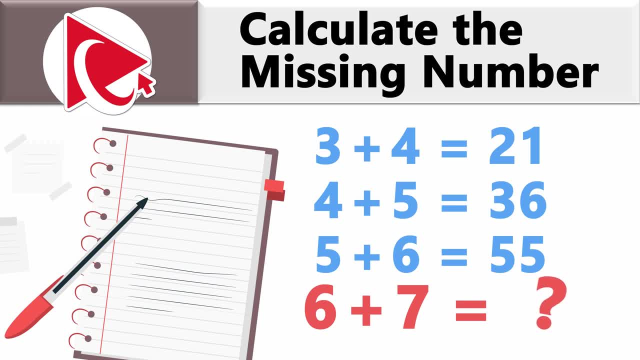 96., 97., 98., 99., 100., 10. 100., 100., 101., 102., 10. 102., 103., 103., 104., 104., 105.. 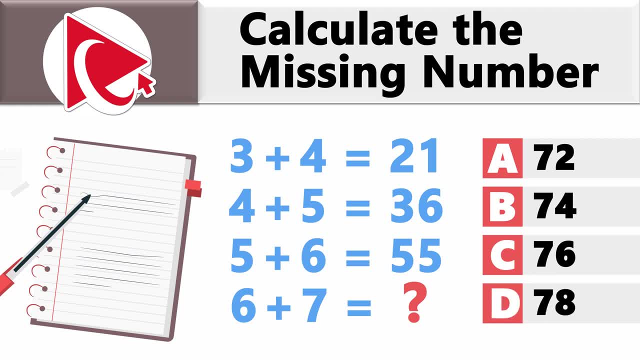 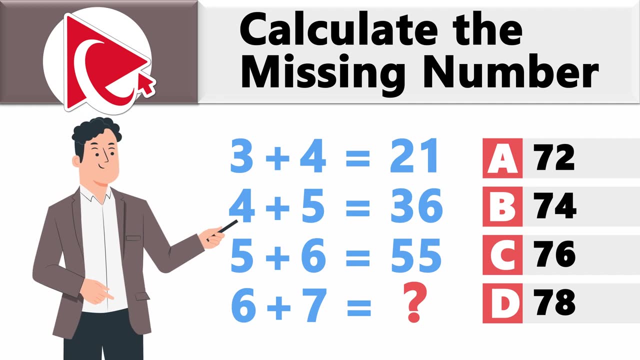 105., 106., 107., 108., 109., 109., 101., 102., 103., 104., 105., 106.. are you ready? let's dive and unravel this challenge together. i'll share with you my solution. 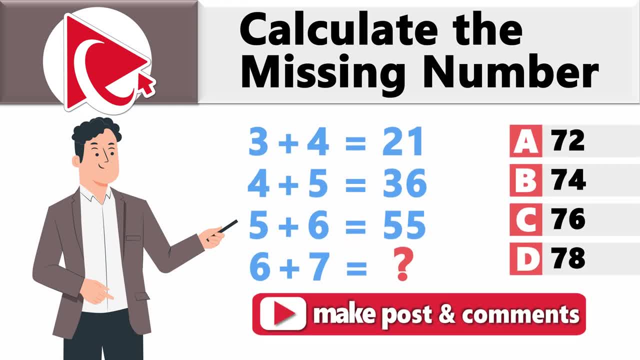 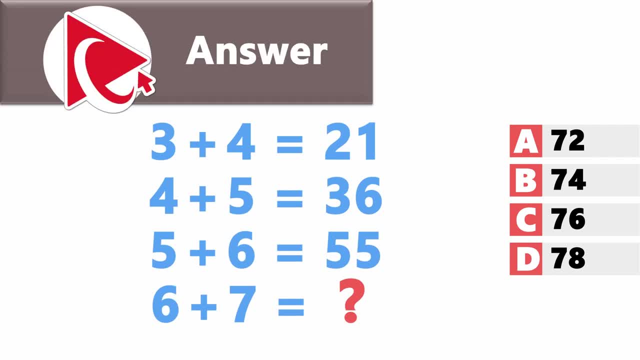 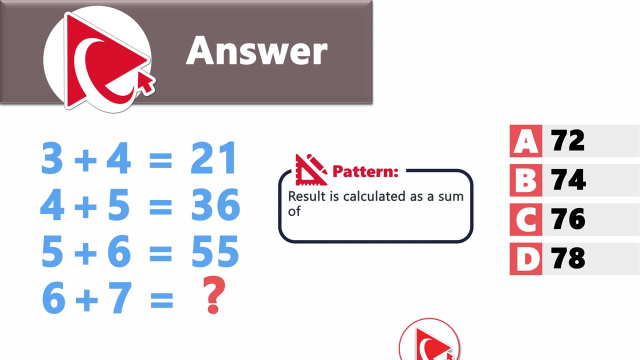 and if you have a better way to solve it, make sure to post in comments. if you are a subscriber or maybe considering to become a subscriber, you probably know that to solve this challenge, you need to always look for patterns, and the pattern here is: the result is calculated as a sum of both. 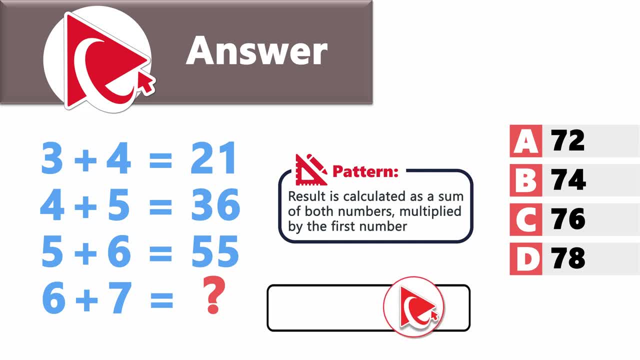 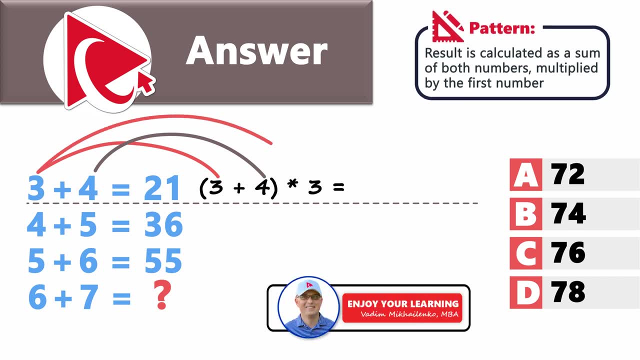 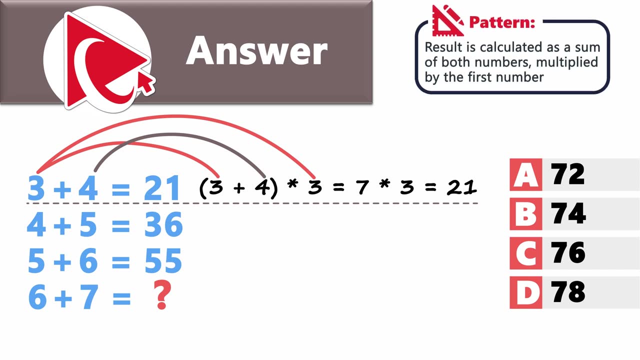 numbers multiplied by the first number. let's look at the example in row one: three plus four equals seven, and then you need to multiply seven by three, which is the first number, and seven by three equals 21. this is how we came to the result. the tip i would like to leave you with to solve these types.